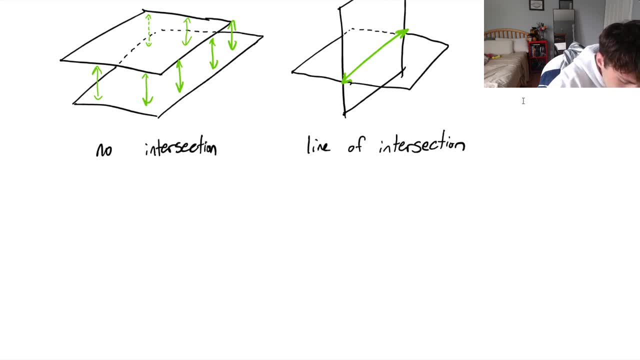 two scalar equations of planes and it's given by 2x plus 8y plus 2z, equals 3.. So this is equation number one for one plane And another. we've got x minus 4y plus 6z, equals 3.. 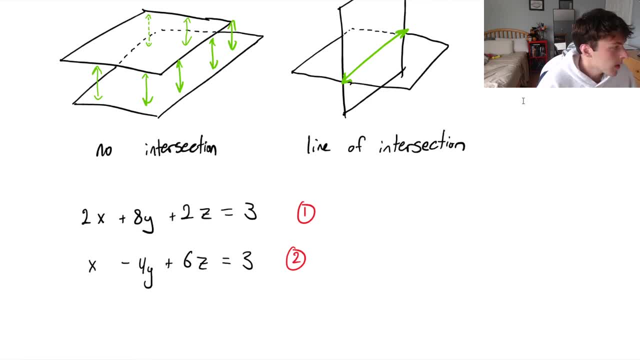 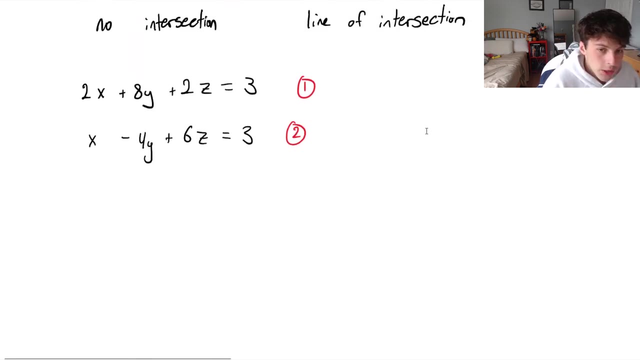 This will be a second equation of a plane And again, this is clearly in R3.. We've got three variables here. Our dimensions in R3 are x, y and z. So in order to find the solutions of the intersection, 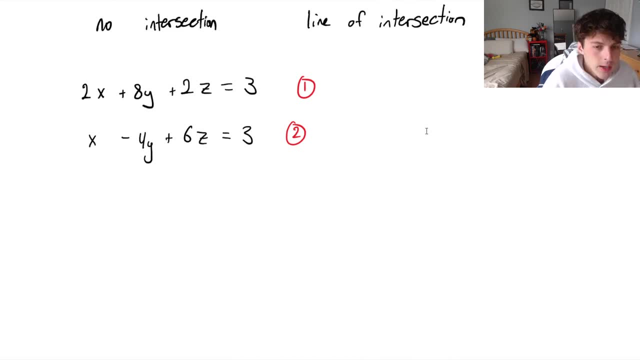 well, same way, if you had like a quadratic, you know If you had two or just two functions. If you want to find out where the intersection is, we need to solve a system of equations of those two functions By equating them and solving that system right. 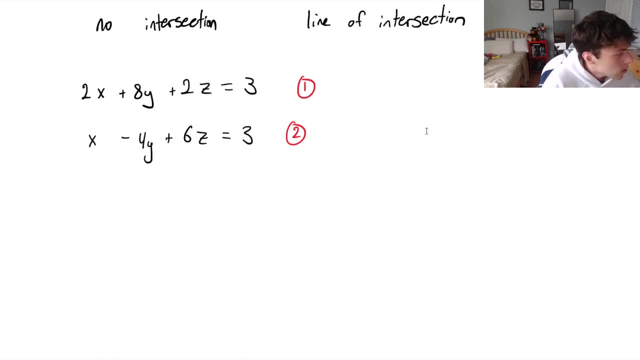 So, similarly, if you have two equations, three unknowns, we're just solving a linear system of equations, right? So the easiest way to do that, I would say, with this many variables and two equations, is just solving a matrix. 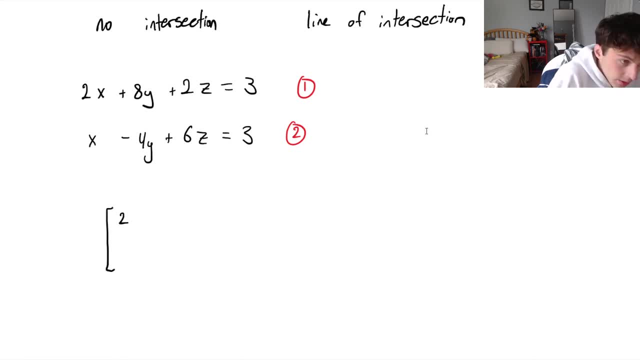 So we could put this into a matrix: 2,, 8,, 2,, and then the homogenous side would be 3, and then, oh x, what am I saying? This should be 1, minus 4,, 6,, 3,. 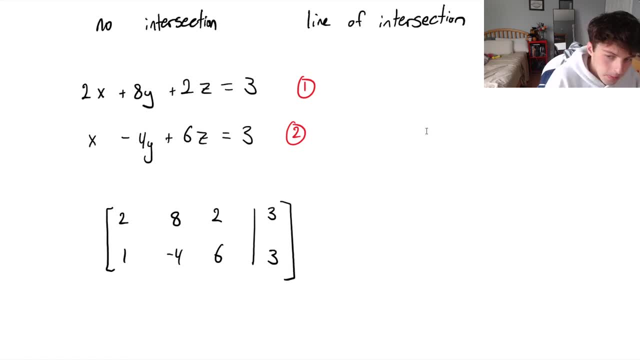 and then we're going to row-reduce this right, So we can fairly simply row-reduce this. So let's do. first of all, let's divide row 1 by 2. Because we want that leading entry in the top left to be a 1.. 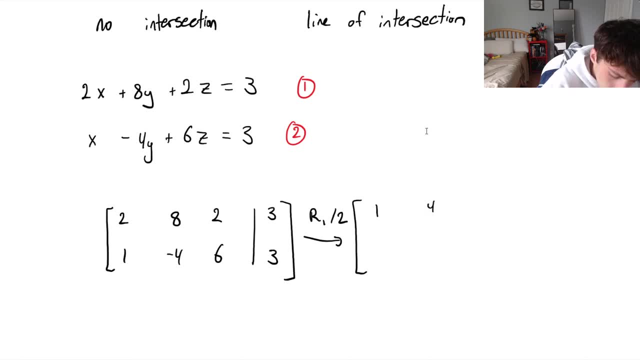 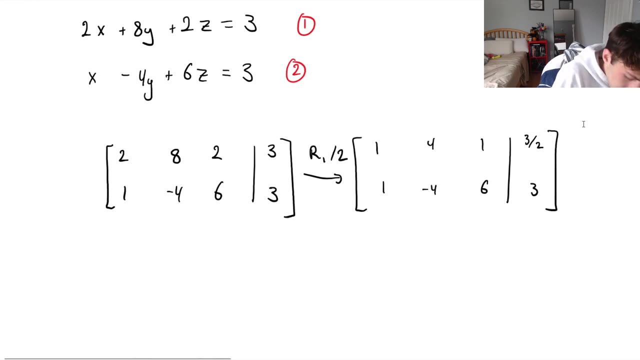 So immediately, let's make that 1,, 4,, 1, and 3 over 2.. 1, negative, 4,, 6,, 3.. Our second row remains unchanged. Let's scroll down a bit, Okay. 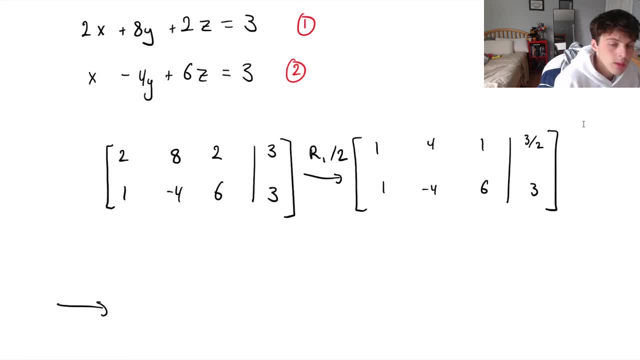 Next, we want a 0 to be in the bottom left entry, right Underneath our leading entry, So we can do row 2 minus row 1.. So 1 minus 1 would be 0.. Negative 4 minus 4 would be minus 8.. 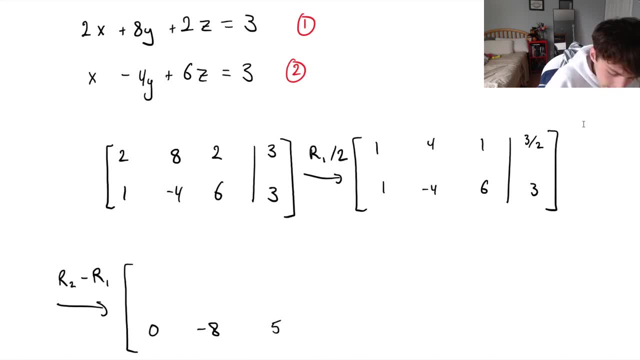 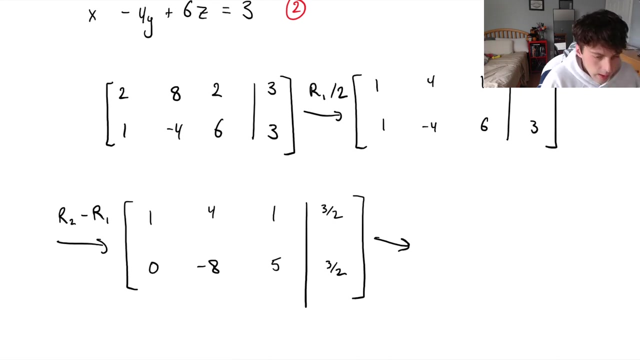 6 minus 1 is 5., And 3 minus 1.5 is going to be 3 over 2, or 1.5.. And our first row remains unchanged. Okay, Next. Well, we, now we have our. that first column is looking good. 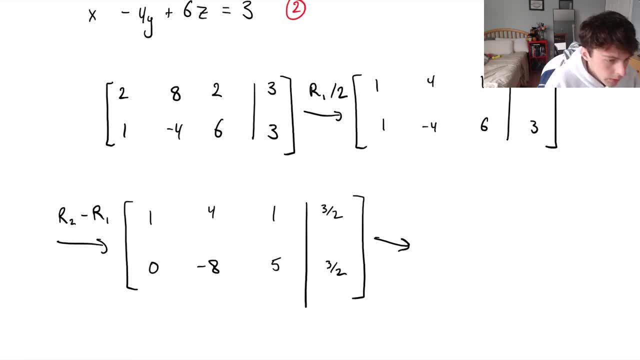 But we want the second column, We need a leading entry to be where that negative 8 should be. So to turn that into a 1, we can pretty easily divide row 2 by negative 8. And that will result in 0, 1, minus 5 eighths. 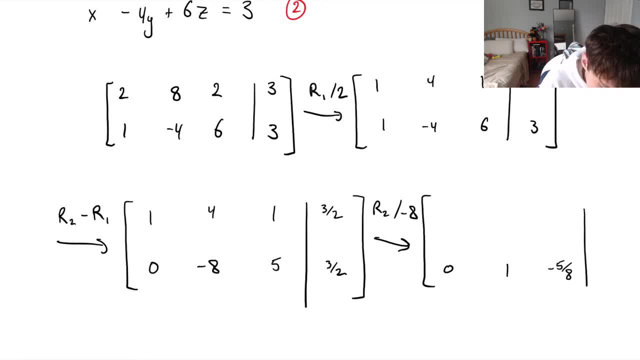 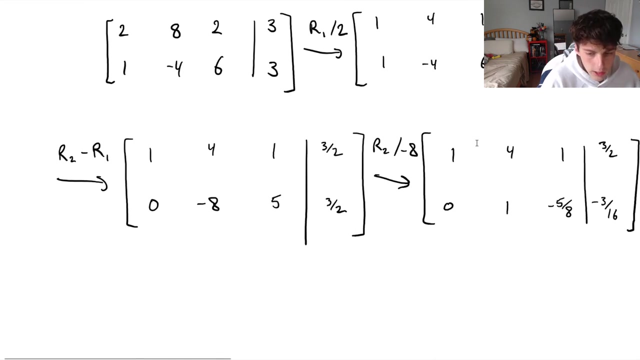 And this will now be minus 3 over 16. And our first row becomes unchanged: 1, 4,, 1, 3 over 2.. And we're getting close. So this is now in REF, right Row, Echelon Form. 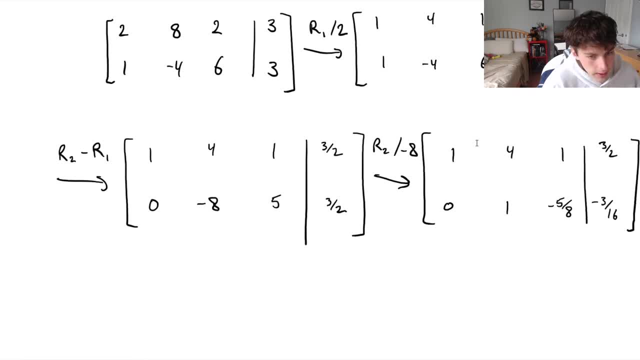 You could write down your new equations, right? Because we've reduced that second column, Or sorry, the second row. We've reduced it by one variable, So it's going to be easier to solve this if you were to rewrite out your equations. 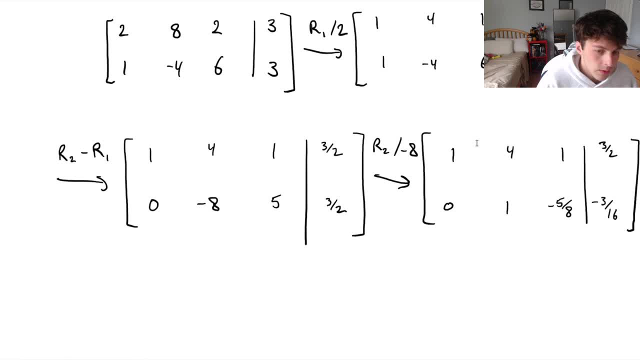 and solve using like plugging equation 2 into equation 1.. It's totally possible to do it that way. It would be a little bit extra work. But what we can do is turn this into reduced row echelon form. It's just going to make our work a little bit easier. 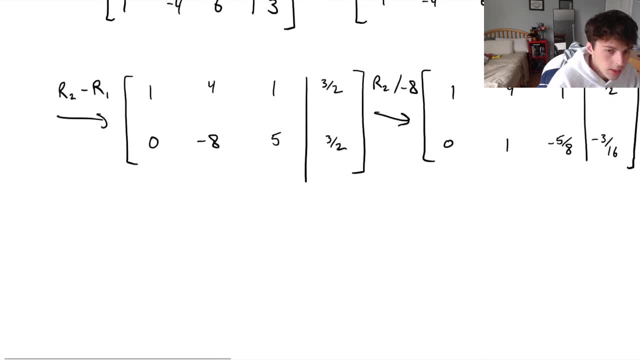 Right, So let's do that, Okay. Next: Oh, that's an ugly arrow. Let's do that again. Okay, So we can do. Well, we're trying to get rid of the 4 above the second leading entry. 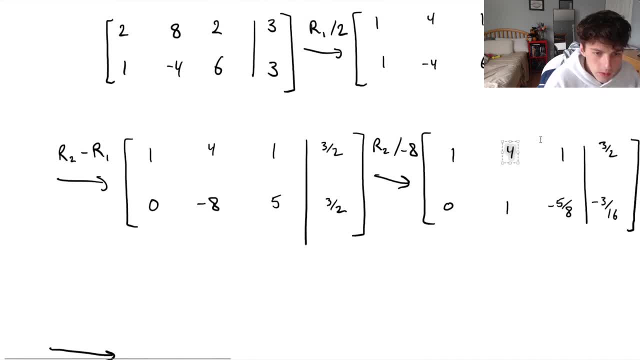 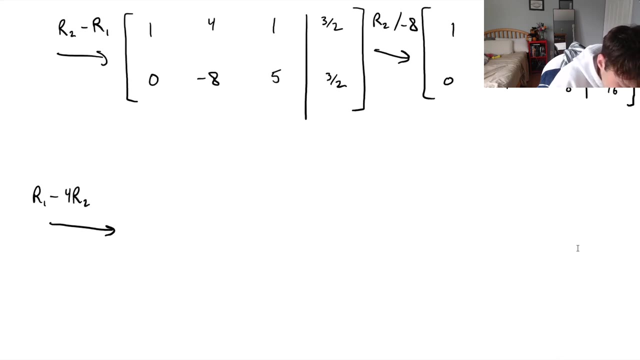 Right, Trying to get rid of this 4 right here, And to do that we could do row 1 minus 4 times row 2.. Right, So row 1 minus 4 times row 2.. So row 1.. 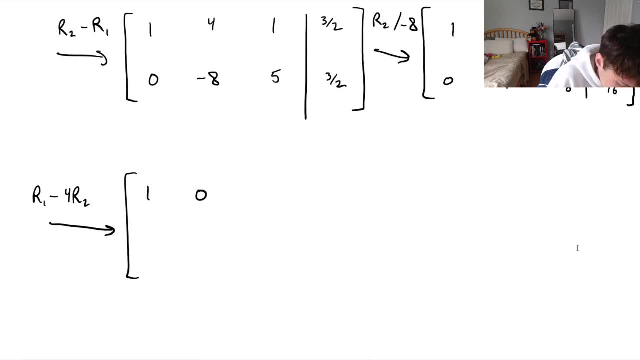 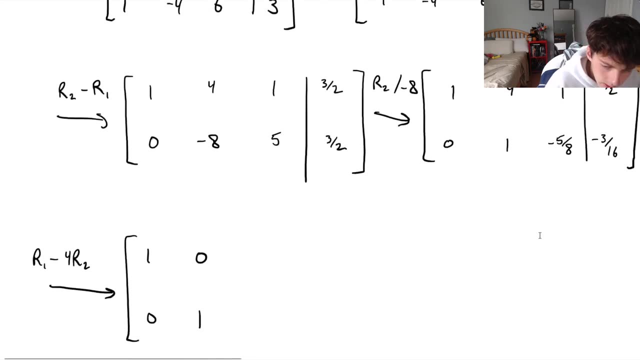 That's 1 minus 0.. This will be a 0.. 0, 1.. And our next entries are going to be a little bit uglier, But it's going to end up in 7 over 2.. And 9 fourths. 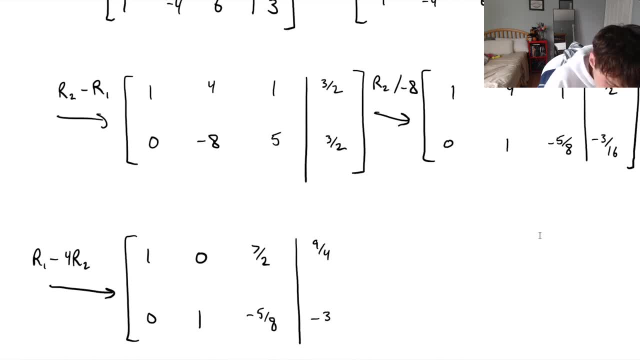 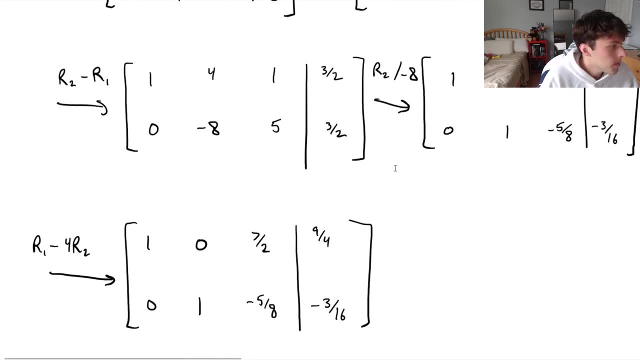 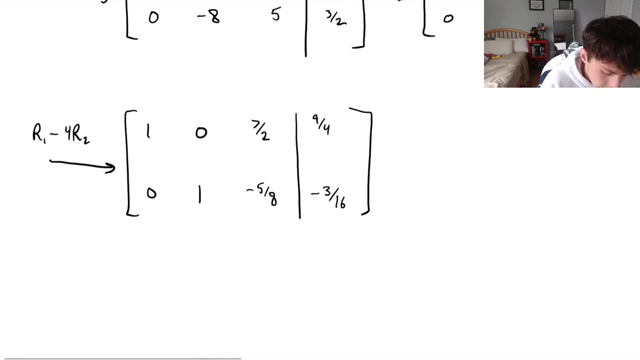 Negative 5, eighths, Negative 3, sixteenths, And now we're finally in reduced row echelon form. Okay, And you can see. now this is a lot easier to write out our system of equations Or the solutions to our equation. 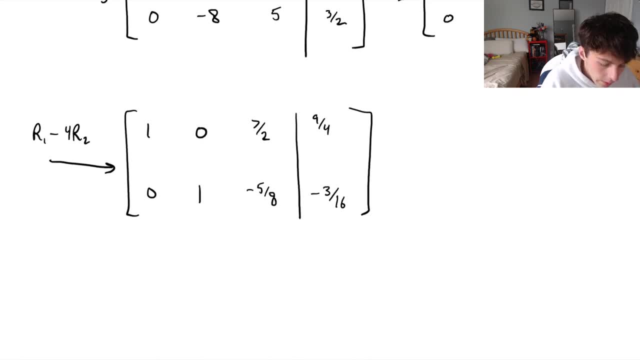 Right, And this totally checks out. Right, We've got one free variable Right, And in this column you can see there's no leading entry, Right? So we've got a free variable here. Totally checks out. We should have one, because we had 3 unknowns and we had 2 equations. 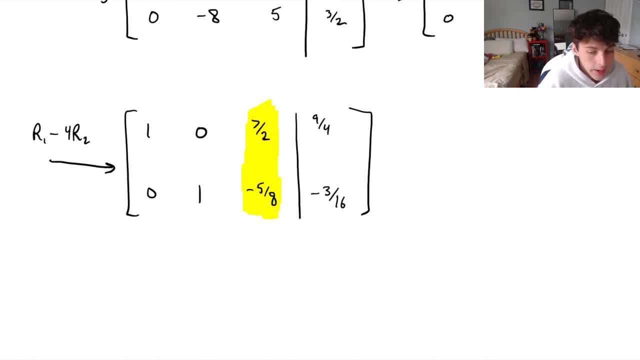 So we need to have one free variable Right. It's impossible to have a unique solution here, So let's write out: Well, we know that this is our Z column Right, So our equations are going to be: 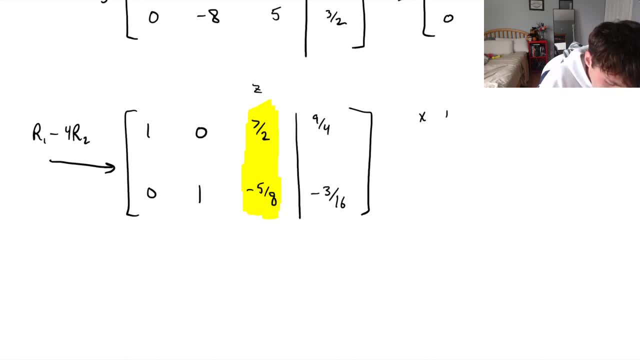 From row 1, we get 1X plus 7 over 2Z is equal to 9 fourths. And from the second row we get Y minus 5 eighths. Z is equal to minus 3 sixteenths. 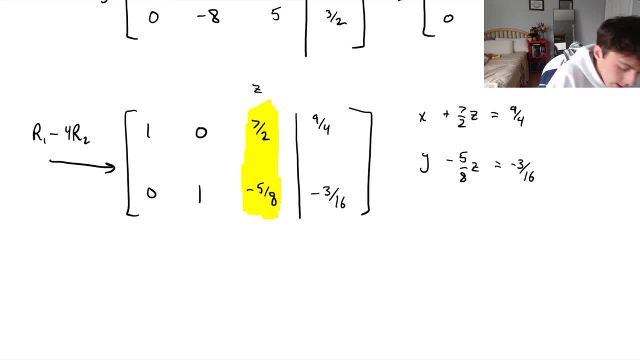 Right, We're reading this directly off of our matrix here, from reduced rational form, Because our first column is X, Our second column is Y, Our third column is Z, And then that vertical line is just that imaginary line and it's kind of representing our equal sign. 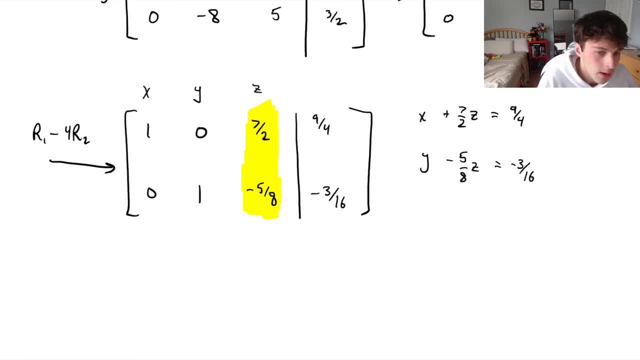 Right, So we're just reading off the rows and turning it back into our Like a similar system of equations. Great, So now that we've got this, Okay, We also know that Z is a free variable, So we're going to write. 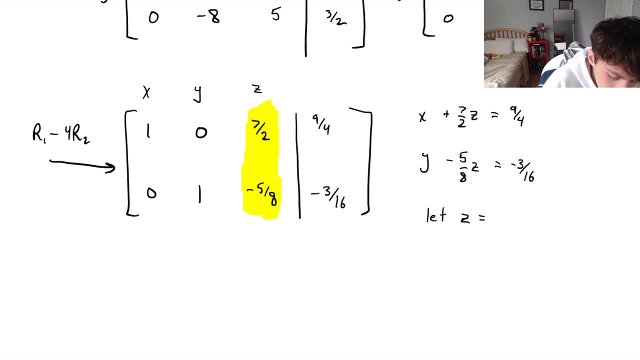 Let's let Z be equal to T. where T is any real number- And this is mostly just convention- T is often the variable that we use to set as a parameter rather than Z, So we're just going to change it to T. 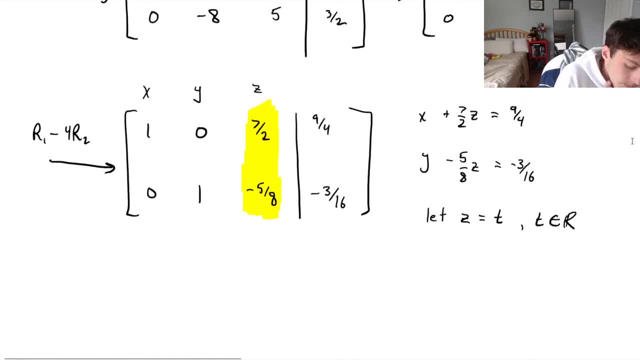 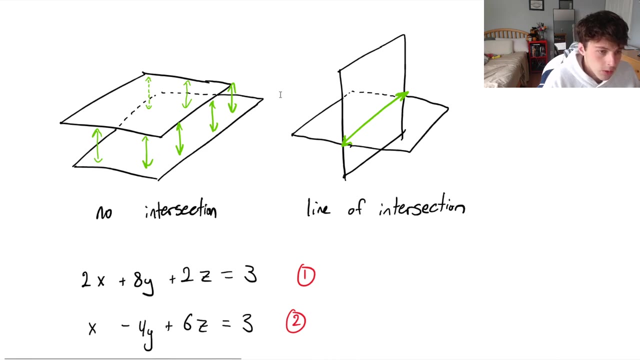 So, okay, You might be stuck here thinking, okay, well, I solved this, But like, how is this an intersection, Right? So let's look back at what we're looking at here. We found a solution, right? Or it looks like there is some solutions that exist. 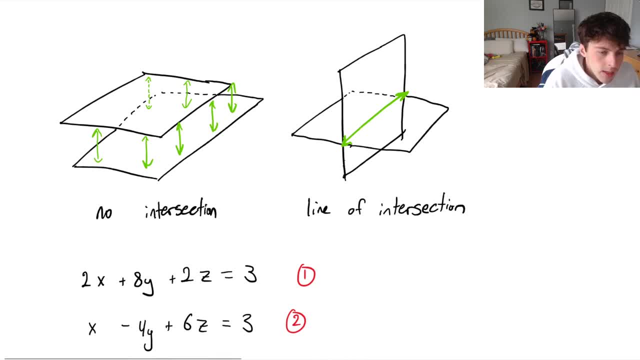 And it's going to look something like a line, Right? Because they're planes, They extend infinitely, So we should have infinite solutions that are represented by some line, Right? So the best way to represent our answer would actually just be a vector equation of a line. 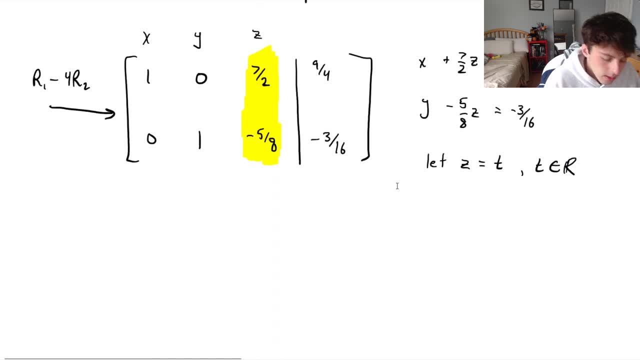 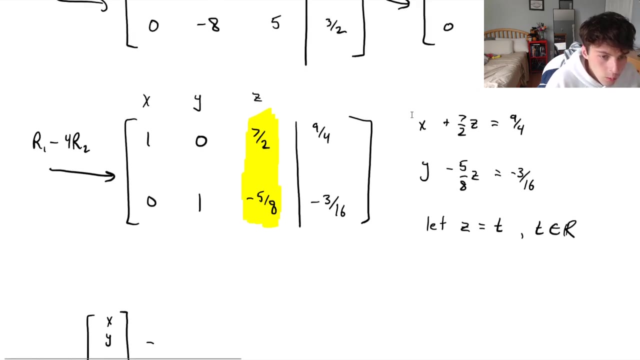 So let's start by writing out a vector equation of a line Right: X, Y, Z would be equal to: Well, okay, What is X? Okay, Well, we can rearrange for X. right. here We have 9 fourths minus 7 over 2 Z. 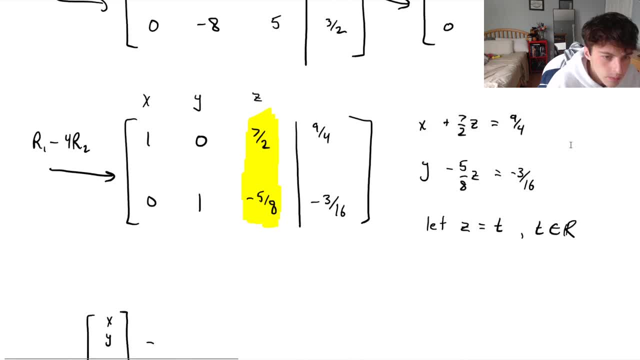 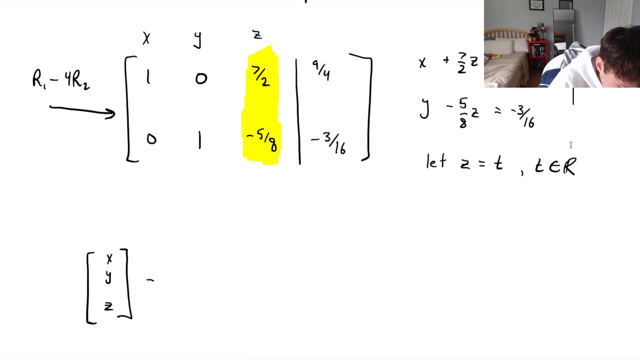 Right From right here. So we can say: X would be equal to 9 fourths minus 7 over 2. Z- Right, I'm just replacing the X entirely, Right Y. similarly we could do minus 3 over 16.. 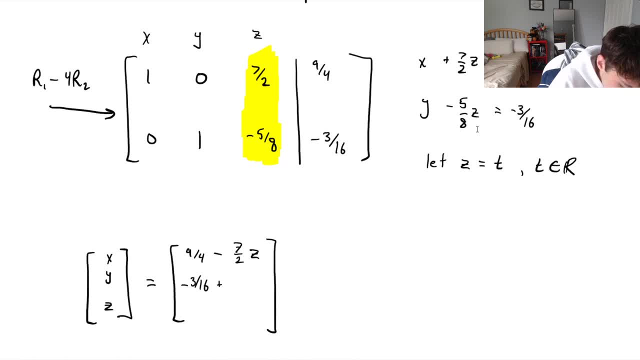 And then we can move the 5 eighths Z to the other side, Plus 5 eighths Z, Great And Z remains unchanged. Okay, And now you can see here we can actually break this up. So we've got this first vector here.